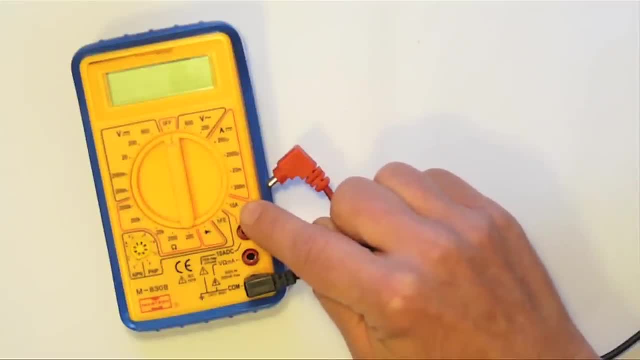 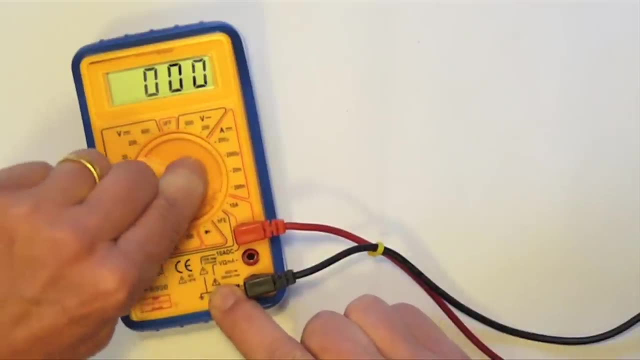 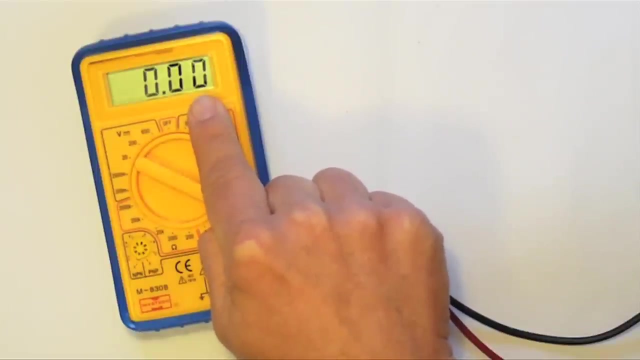 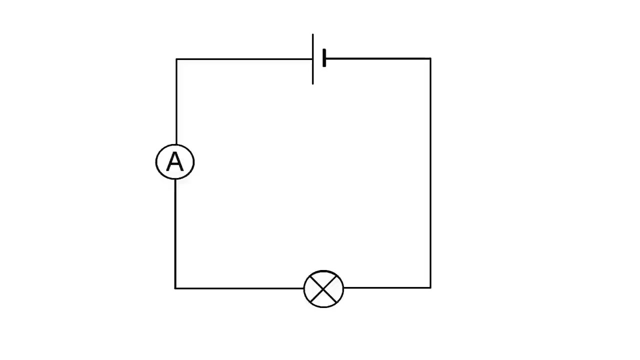 on this setting. lets me measure currents up to 10 amps, but nothing smaller than a hundredth of an amp. If you go above 10 amps you could destroy the multimeter. Let's measure the current in this circuit. Ammeters are always connected in series. 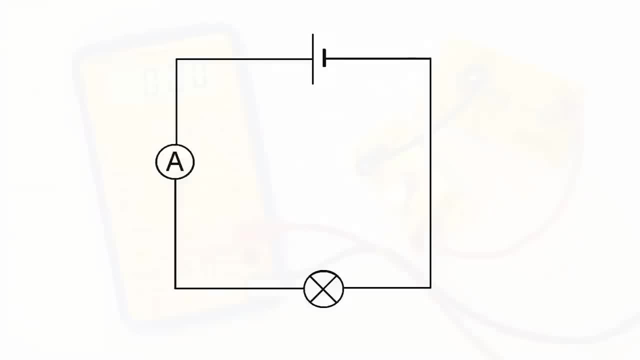 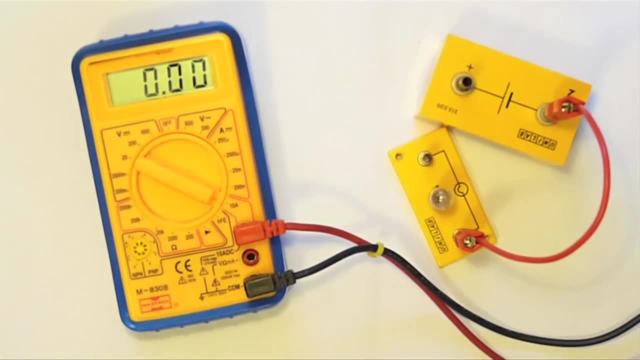 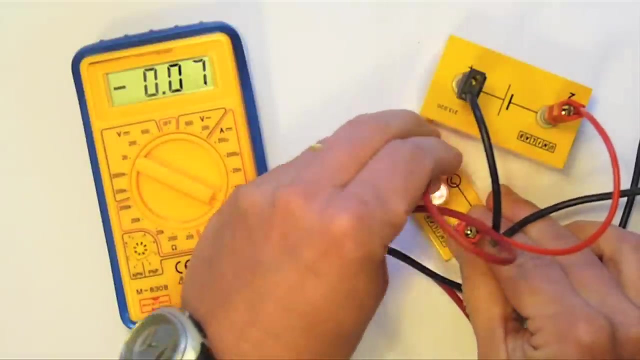 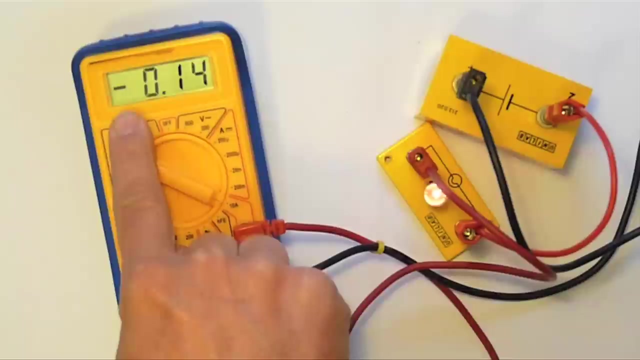 so I need to break the circuit and then complete it again with the ammeter in series. The minors just means we have the opposite polarity: 0.14 amps, that's 140 milliamps. Since this is below 200 milliamps, I can measure it more precisely using one of the more sensitive. 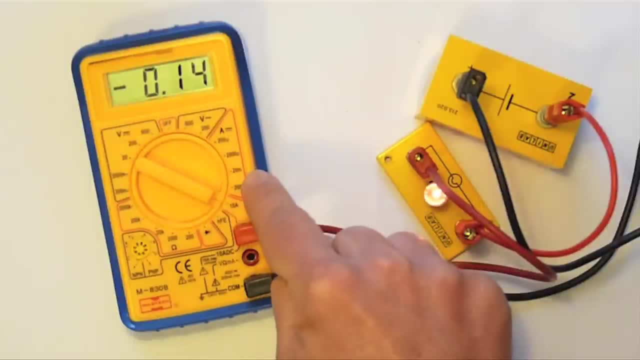 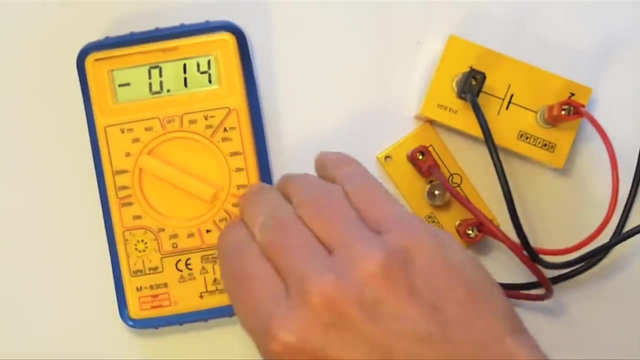 ranges on the on the multimeter. It is a very simple procedure. In order to do this, I need to move the red lead into this socket marked milliamps, which is connected by a fuse which will blow if the current exceeds 200 milliamps. 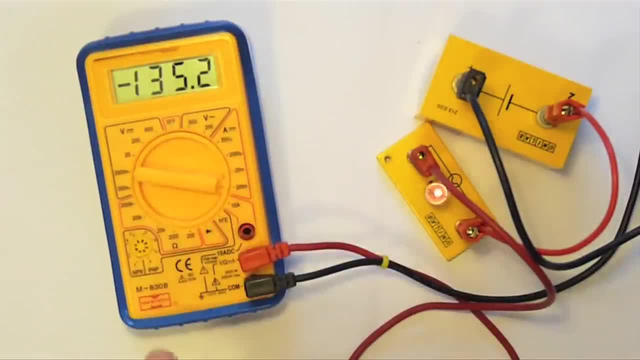 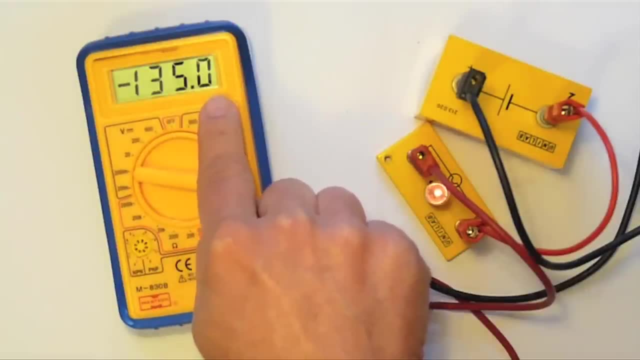 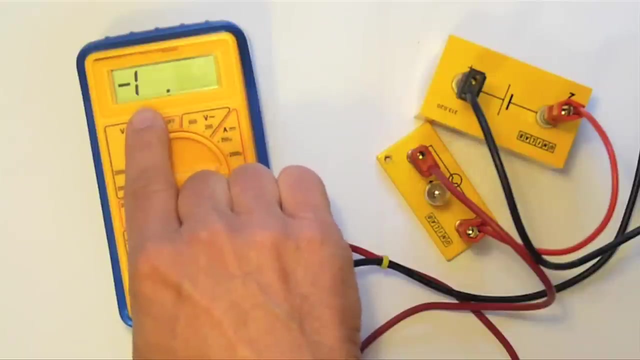 Let's measure the current again: 135.2 milliamps. This is on the 200 milliamp full scale deflection range. If I move to the 20 milliamp range, the current is too high, so I get a 1 on the far left of the display, but there's no harm done. 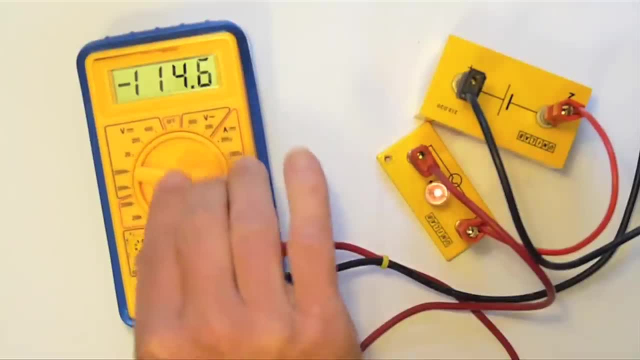 I just click to a higher range to get a reading. The fuse will only blow above 200 milliamps. If the milliamp ranges do not work at all, I just get a 0, then someone has blown the fuse and it needs to be replaced. However, the meter will still work as a voltmeter.